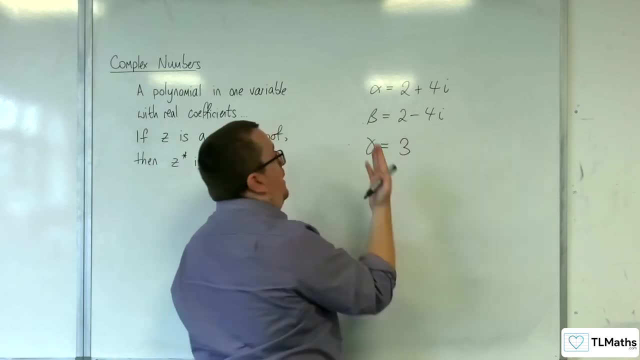 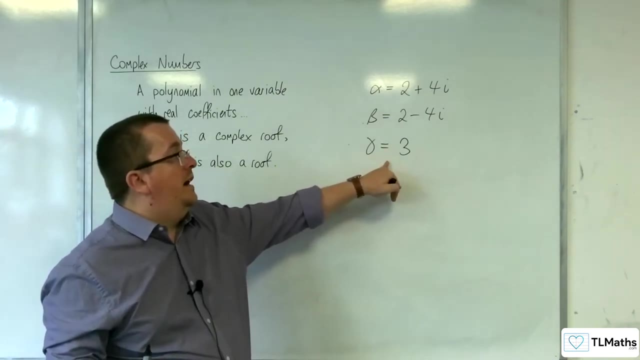 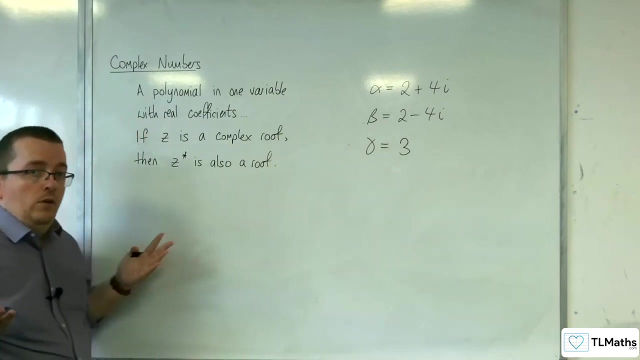 So let's say gamma is equal to 3.. So it has three roots. Okay, But the third root is going to have to be real. Okay, Because I can't have a third root. that is a complex number, Because otherwise you don't have the pair to go with that other one. 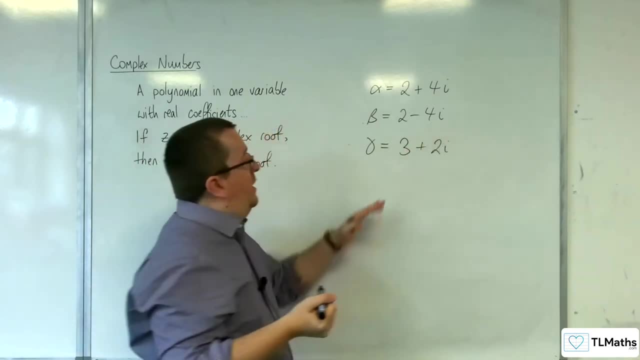 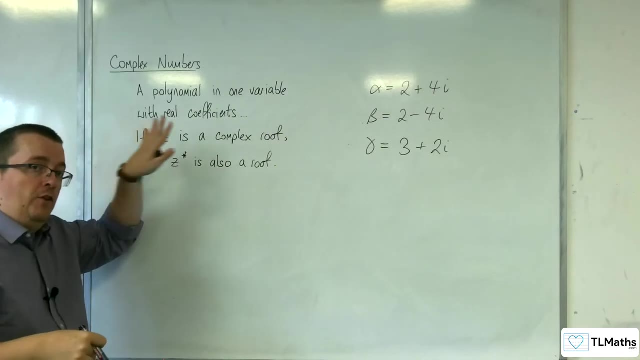 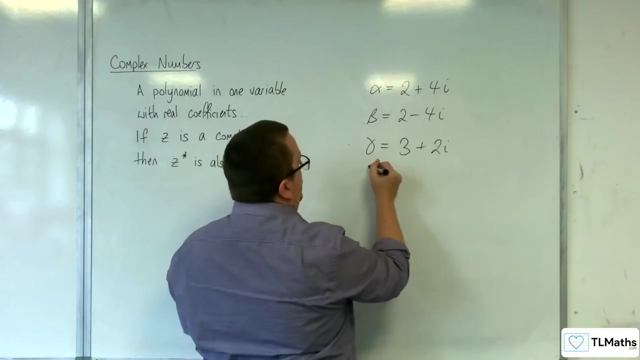 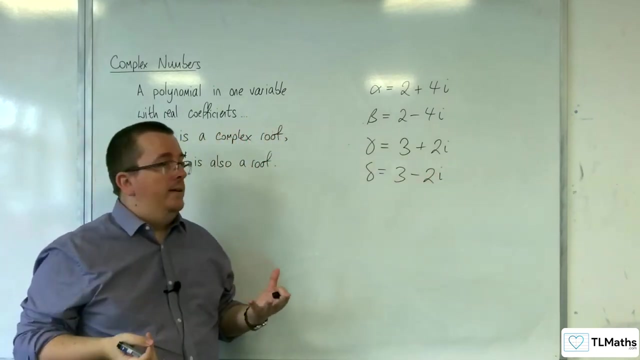 So I can't have like 3 plus 2. Because the complex conjugate- well, sorry, the complex number roots have to appear in pairs because of the complex conjugate root theorem. So if we had 3 here, then I would need to have, let's say, delta. I would need to have another root, that is, the complex conjugate pair. 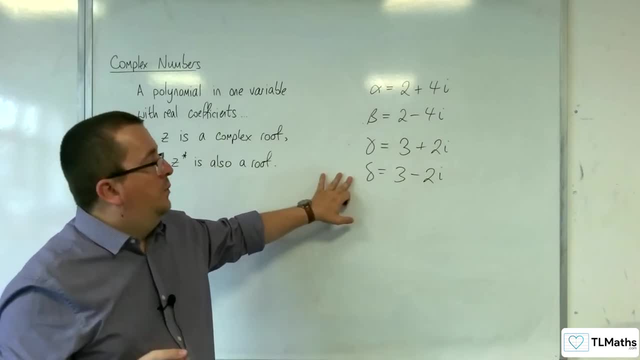 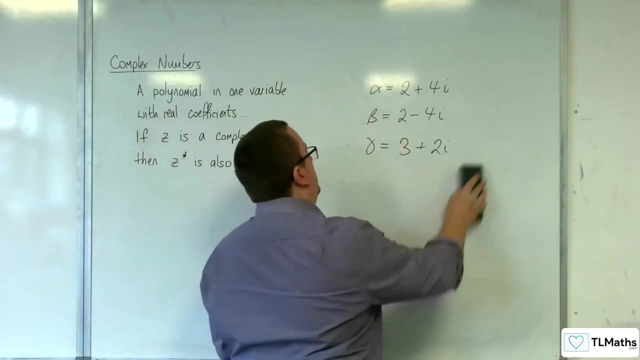 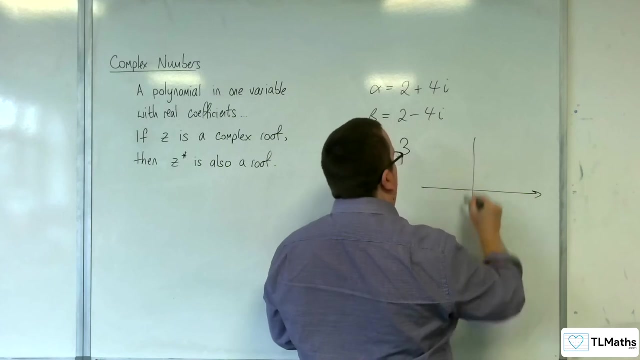 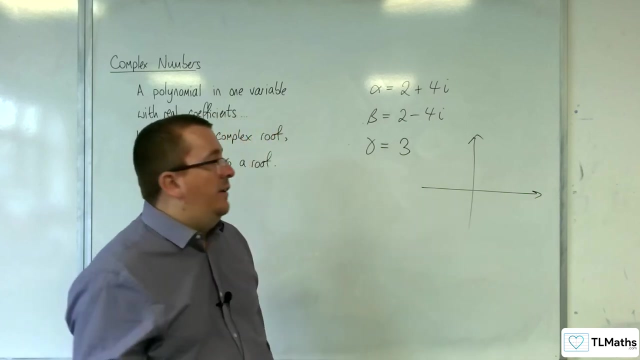 So now I would have a quartic. Okay, Now another practical reason as to why you're A cubic would have to have at least one real root is that because when you draw a cubic right, if it's a positive cubic, so x cubed rather than a minus x cubed- it's got to start in the bottom left and work its way to the top right. 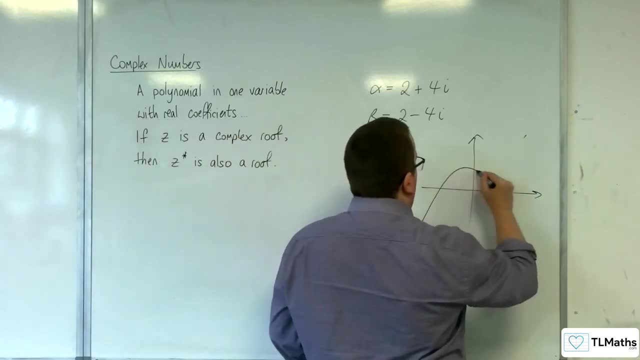 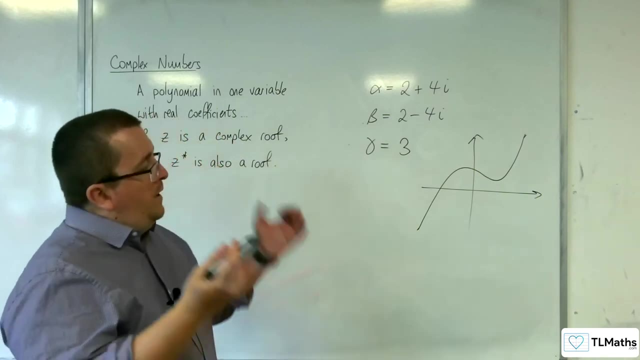 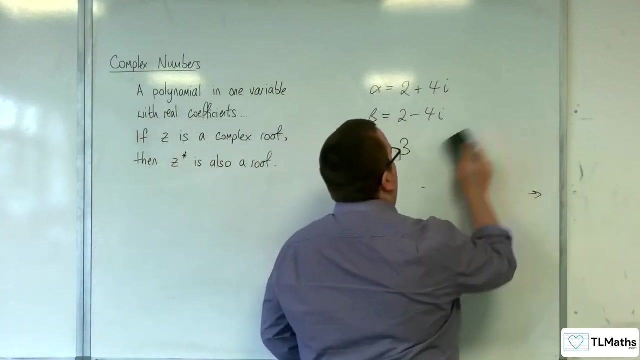 So at some point it's got to cross the x axis. So it will have. It will have to have a real root. There's no way that you can have your cubic and it not cross that x axis, While if you do go for that quartic- so 3 plus 2i and delta is 3 minus 2i- it's perfectly fine for a quartic. 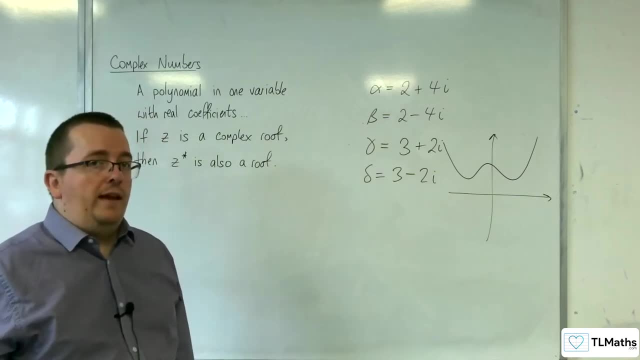 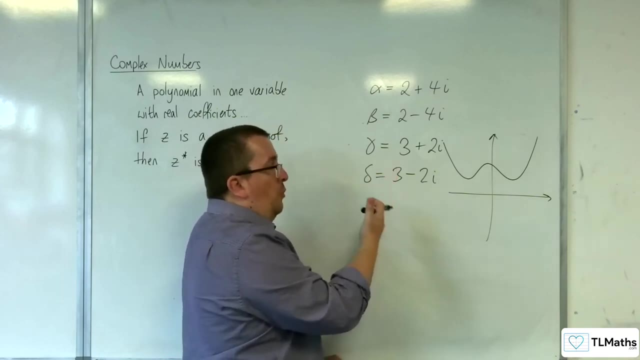 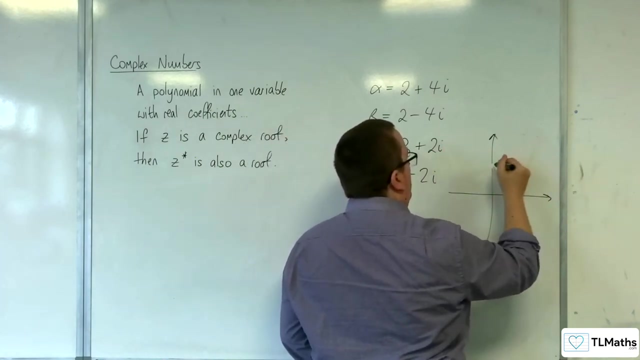 Okay To look something like that and never cross the x axis, But then if you had another root in, It's going to have to be real for a quintic, because for a quintic it's got to cross the x axis at least in one place. 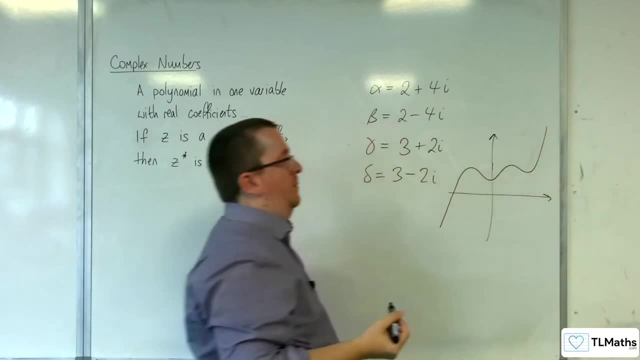 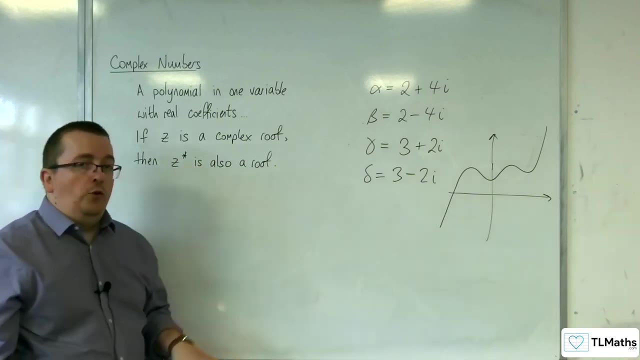 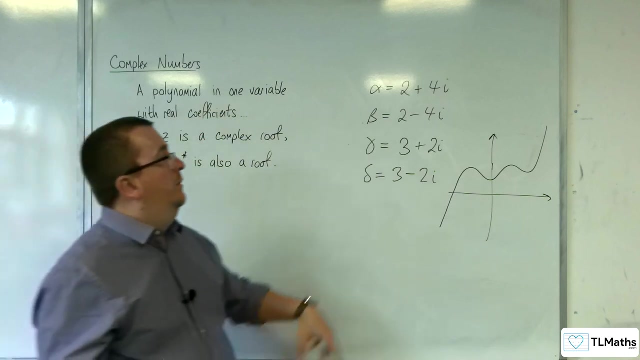 So one could look like that, for example. So this is a very useful, important theorem, Okay, That you can utilize, because if you know one of the roots is complex, You automatically know it's complex. conjugate has to be a root as well.